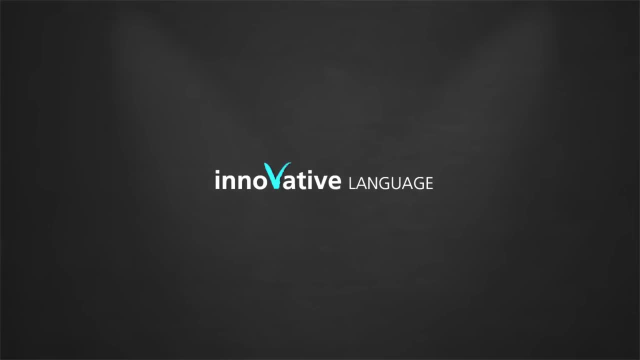 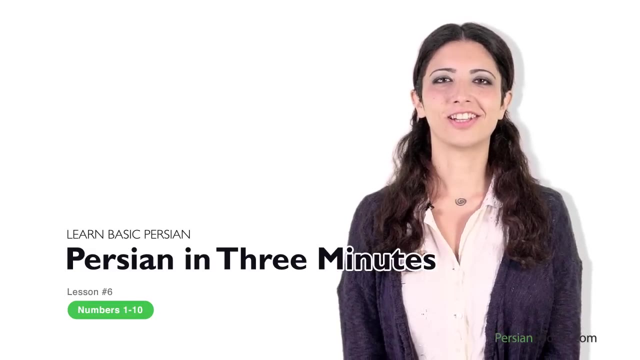 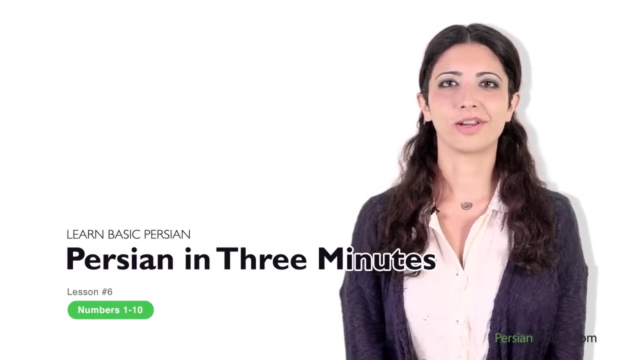 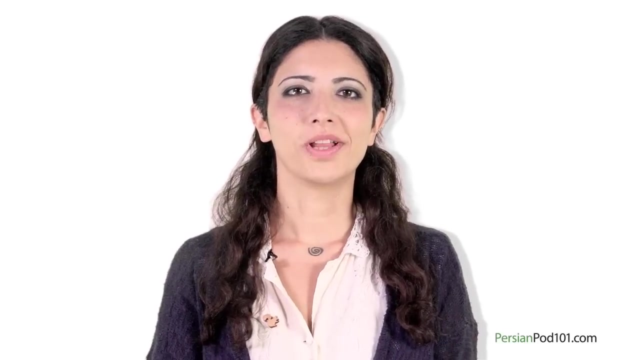 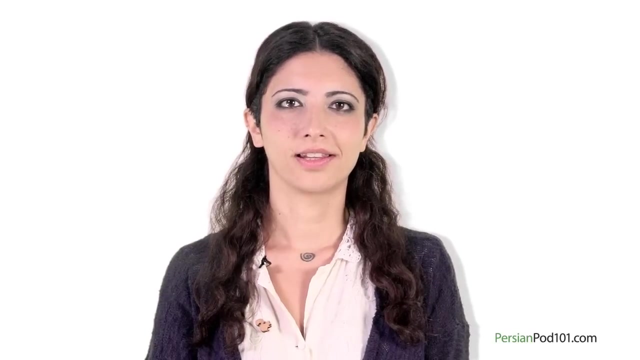 Hi everybody, I'm Anita. Welcome to PersianPod101.com's. Persian in 3 Minutes- the fastest, easiest and most fun way to learn Persian. In the last lesson, we learned some words used when apologizing in Persian, including bebakhshid and lotfan. In this lesson, we are going to learn numbers. 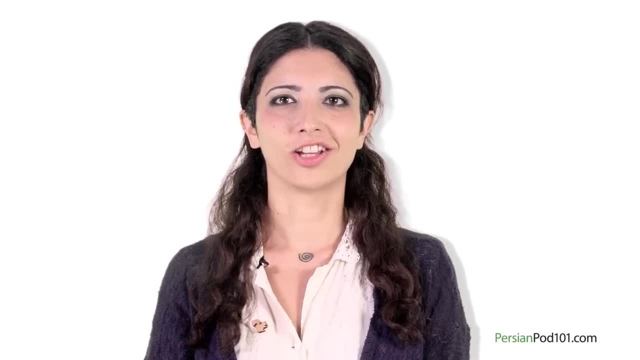 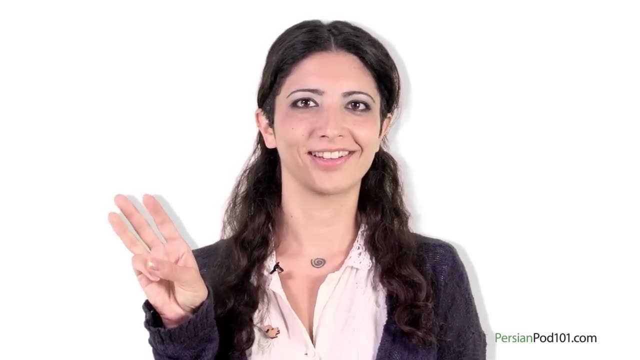 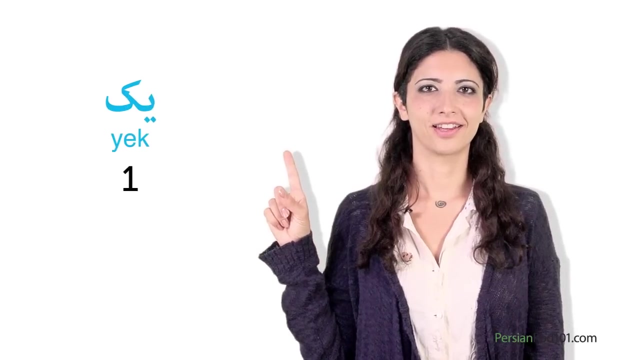 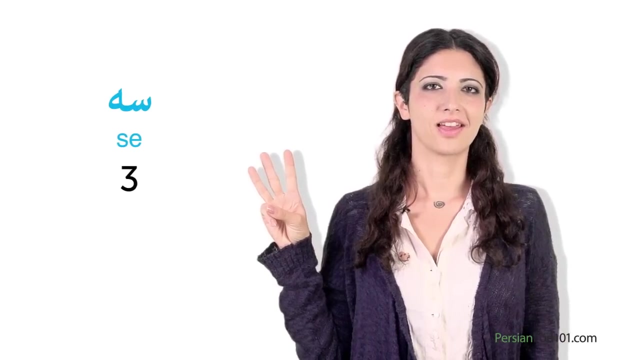 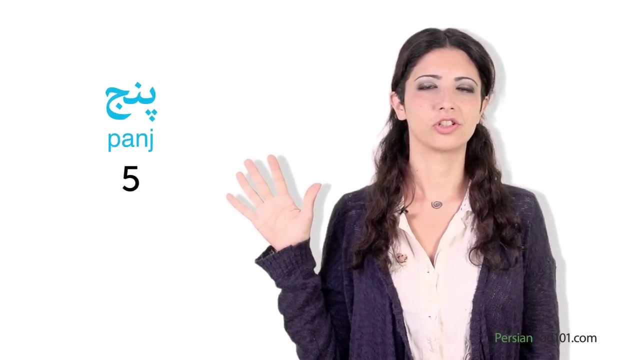 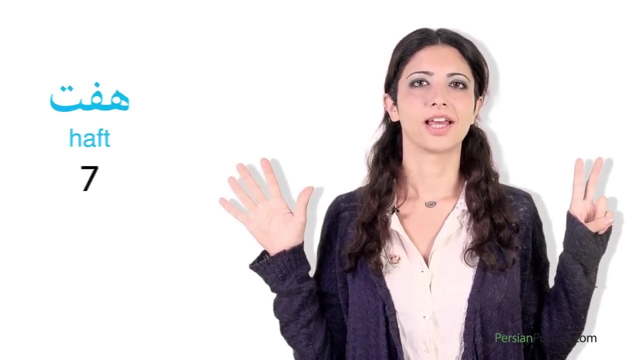 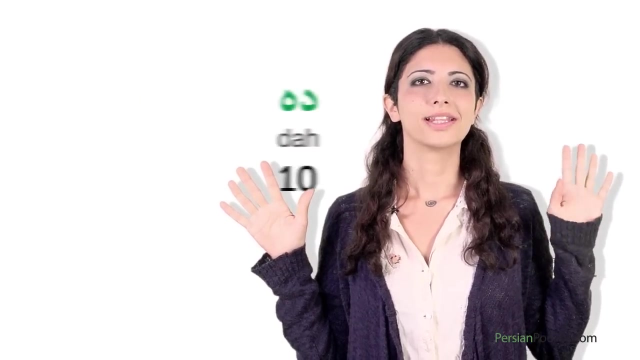 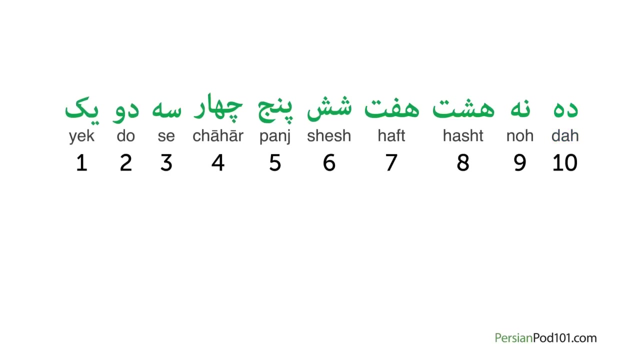 in Persian. Yes, numbers Adad from 1 to 10. And you are going to learn them in only 3 minutes. Are you ready? Let's start? Okay, now repeat after me. I'll say the numbers and give you time to repeat each one. 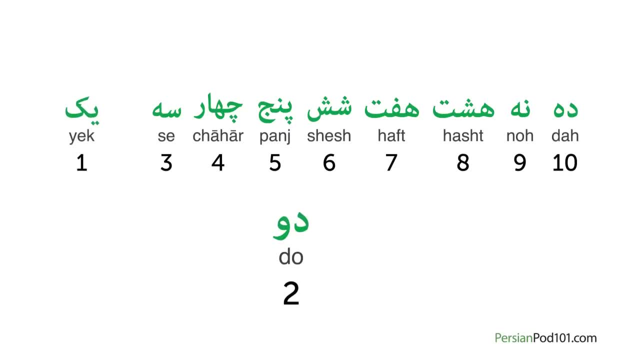 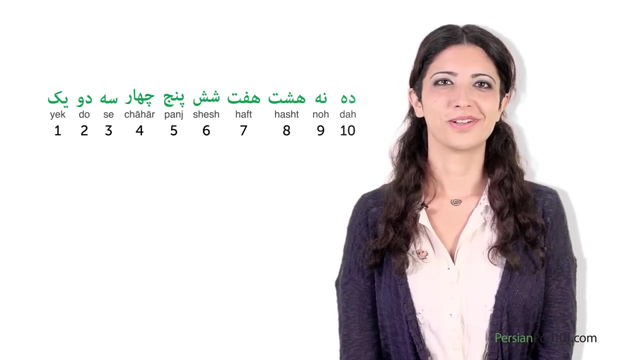 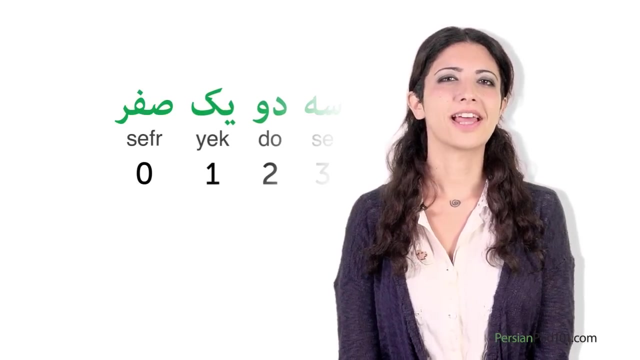 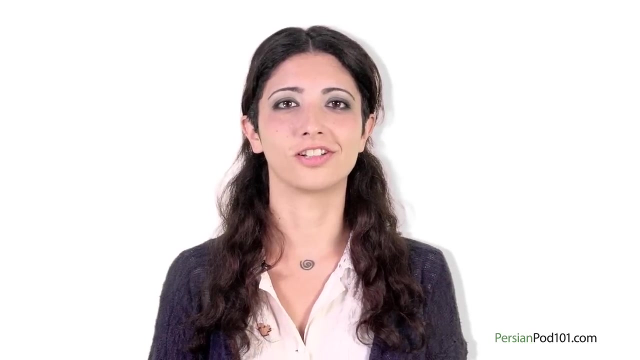 yek do se chahar panj shish haft hashd noh, noh, tah. Great job. What is before? yek Do you know? It's sefsh Sefsh. You don't have any more excuses. You can give your friends your cell phone number in Persian. Let's try. 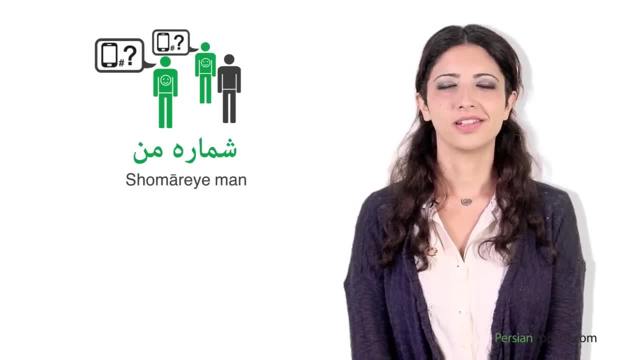 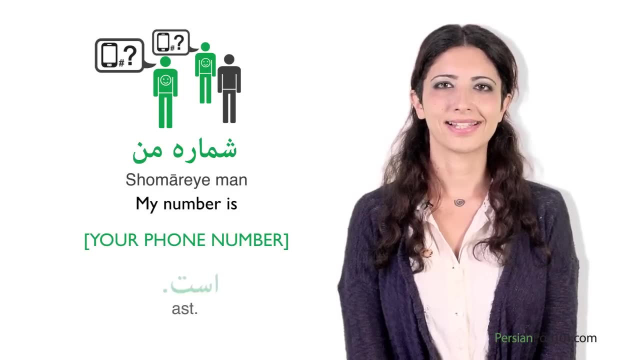 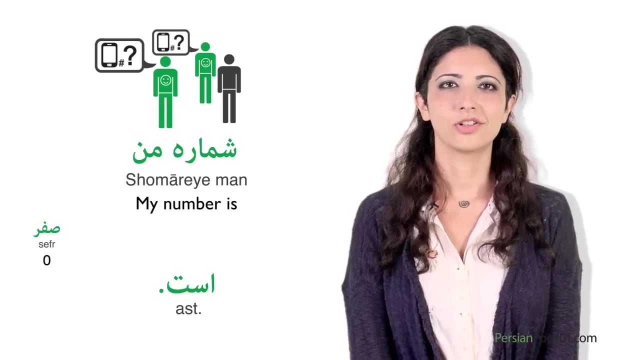 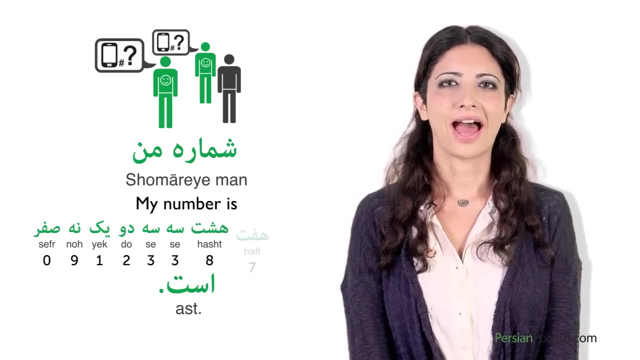 it together. We'll use the phrase shomareyeman, which means my number is. You say the numbers after that And then finish by saying: ast shomareyeman, ast shomareyeman, sefsh noh yek doh se se hashd haft chahar panj ast.